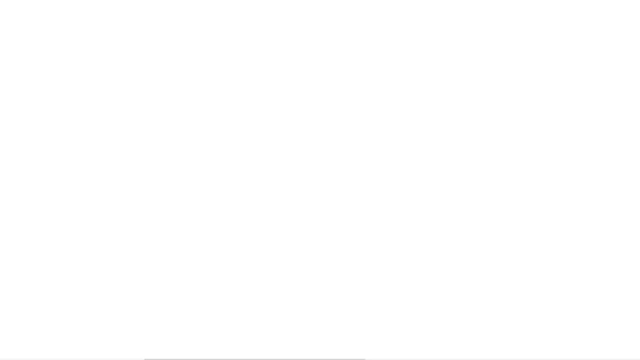 examples of this is the proton acceptance of ammonia to form an ammonium ion and the proton acceptance of a H plus ion by H2O to form a H3O plus ion, and I'll draw up what these would look like. So when NH3 is exposed to acid, so NH3, and that's basically a nitrogen bonded to a hydrogen. 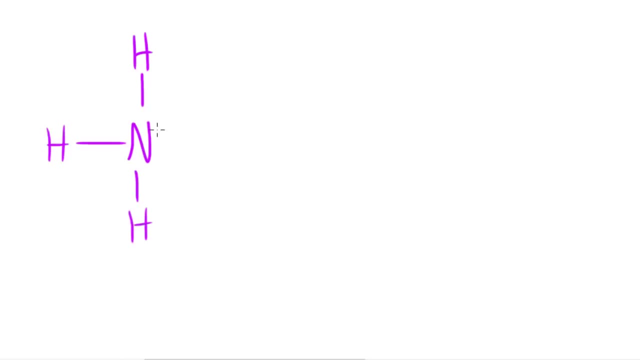 bonded to a hydrogen. bonded to a hydrogen and the nitrogen in the middle has a lone pair of electrons when this is in the presence of acidic conditions. so there's H plus ions in it, certain concentration in that substance. what happens is this NH3 molecule will accept a 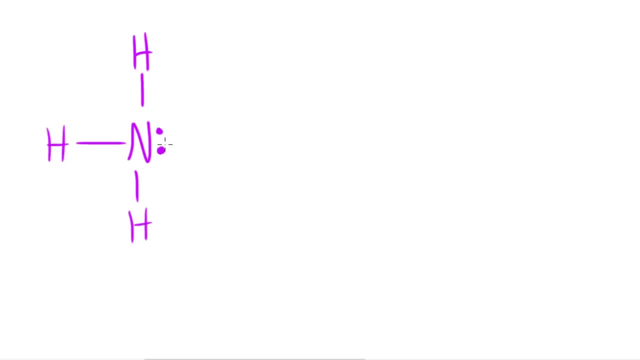 proton, and the way it accepts the proton is by donating a known pair of electrons. So what will happen is – my last video – what would happen is if I represent this nitrogen with a circle, what will happen is the H plus ion will come along and it will actually 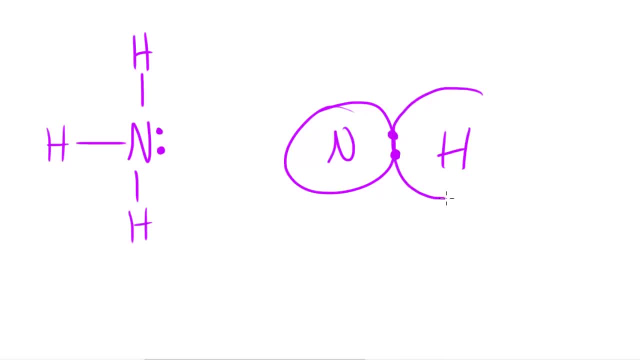 accept – the electrons will be donated to the H plus ion, and when this happens, the nitrogen doesn't actually let go of them, but what it basically does is it's basically saying to the hydrogen: come over here, Okay, Okay, Okay, And we'll share. 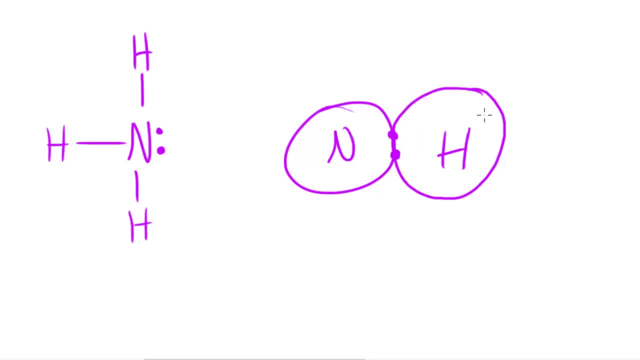 Now, the reason why this happens is because hydrogen ions are really positive. So H plus ions are really really positive. H plus H plus, They are really really positive. and the known pair of electrons which you can see here are quite negative. so, if you remember from ionic bonding, they're caused by the attraction. 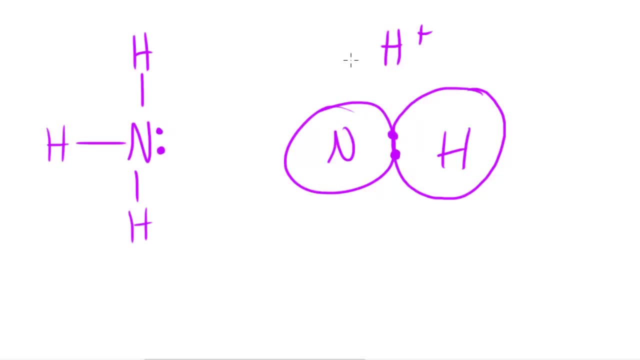 between oppositely charged ions. In this case, what happens is this positive ion? there's an element of natural 있잖아요. positively charged ion is attracted to the negative lone pair of electrons which you can see here. So when they come together they form a covalent bond, just like these. 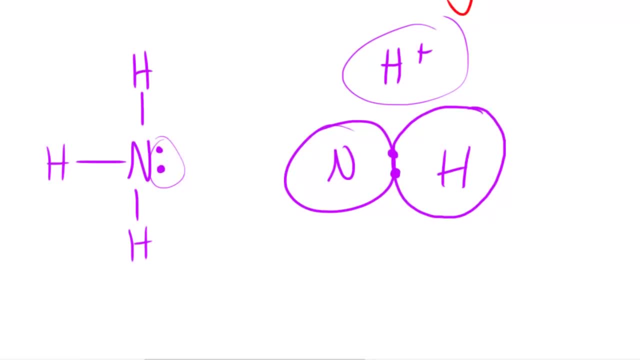 other covalent bonds. So there's a specific notation we use sometimes to represent this kind of bonding and we use lines and we use arrows. So with this NH3 molecule forming an NH4, what we would do to represent it is we'd have the nitrogen we'd use square. 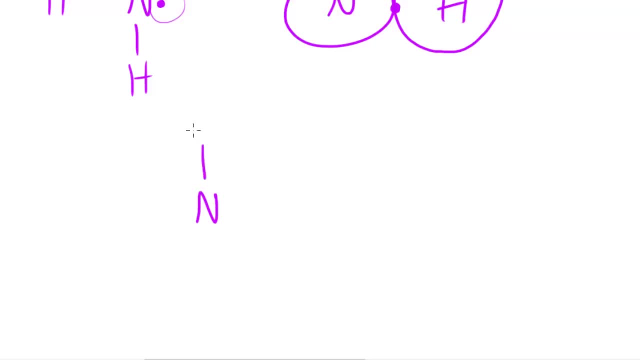 brackets, just like we use in ionic bonding, and we'd have the regular bonds, So the regular bonds here, And then we'd actually have an arrow pointing to the fourth hydrogen. And the reason why we have that arrow there is to represent that both of the electrons in 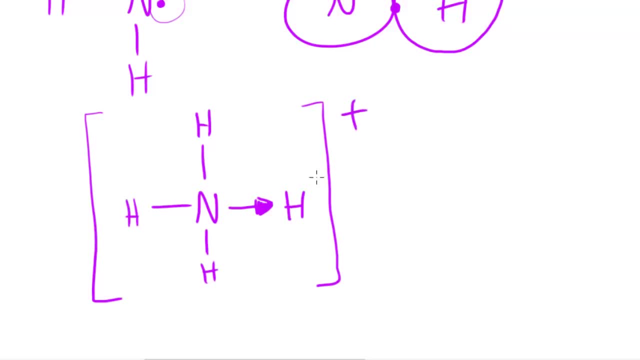 that bond has come from the nitrogen. Okay, So that means that it is a dative covalent bond or a coordinate bond, And this is how we represent it, And we wouldn't make sure you don't if you were writing this, don't. 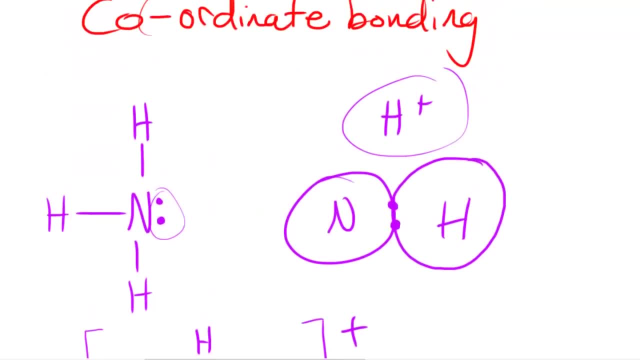 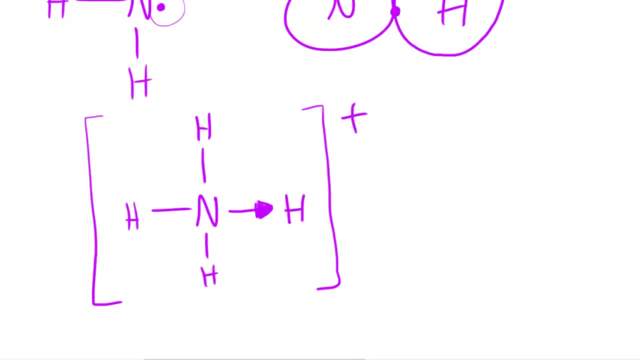 forget the positive charge, because this hydrogen has added to the positive charge of this particular molecule because it was just a proton. And there's also another kind of notation we can use with this. We can use the dot and cross notation. So what we can do is represent. I'm going to use a blue and a blue and red. 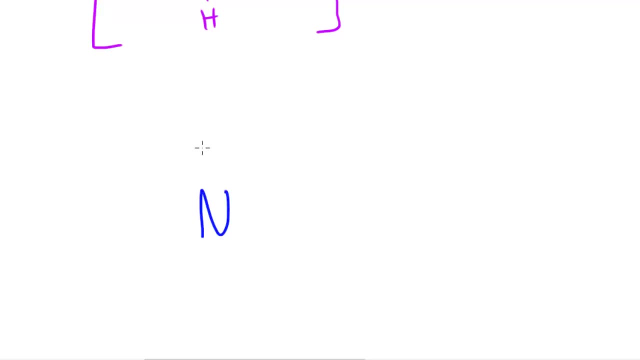 for this. So we have the nitrogen and we have the hydrogens. So hydrogen, hydrogen, hydrogen, hydrogen. Okay, Okay, Okay, And still with the square brackets and the positive symbol. here What we have is the if I represent the nitrogen's electrons with a blue dot. so a blue dot, blue dot, blue. 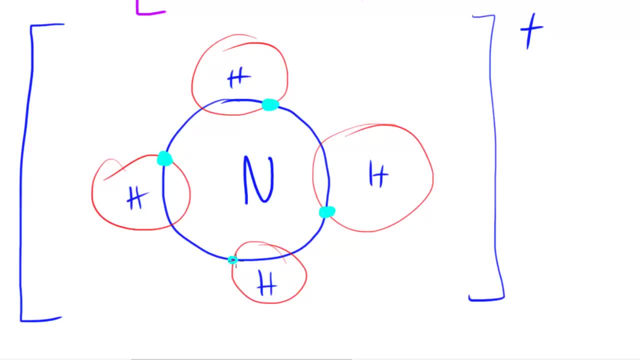 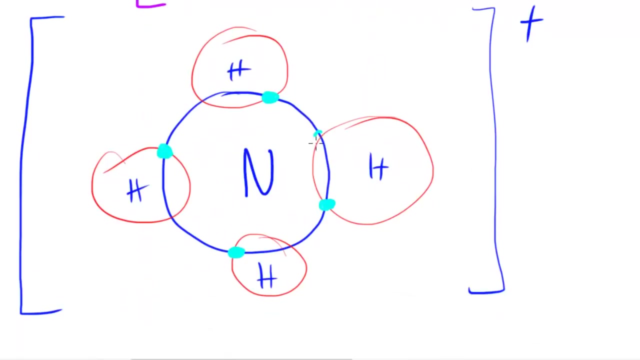 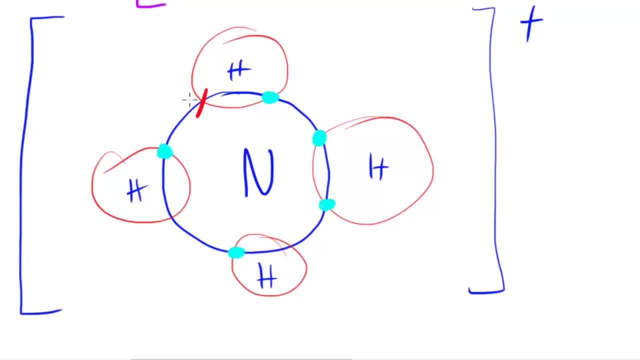 Okay, Okay, Okay, Okay, Okay, Okay. As you can see, only three of these electrons have come from the hydrogens. In this one, this is the dative covalent bond. So this notation is basically showing us that this is the dative covalent bond. 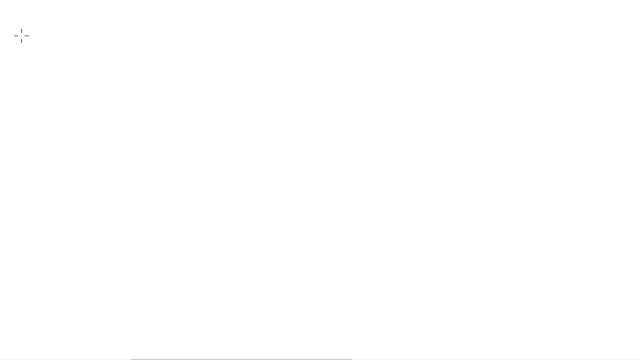 Now a more common example, one that you'd see if you have any sort of aqueous acid. what happens in acids is that, although we usually say that it has dissociated and there's a concentration of hydrogen ions, now in the solution what there actually is a concentration. 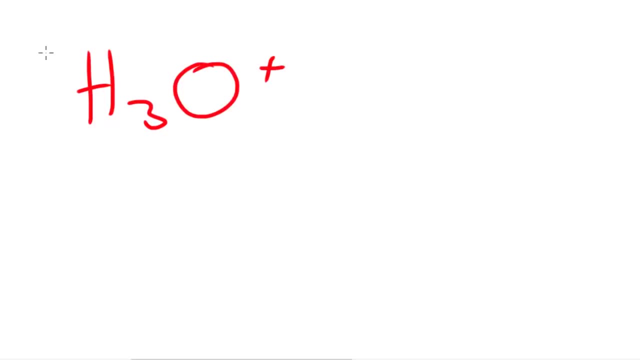 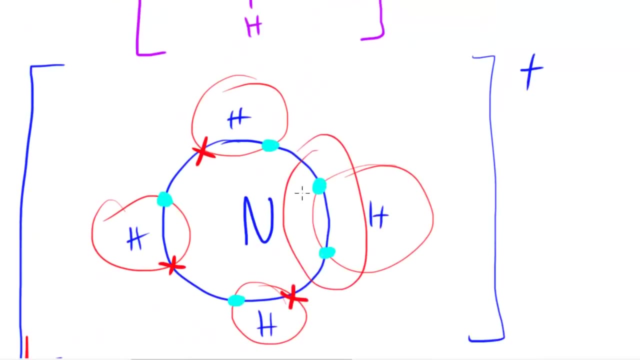 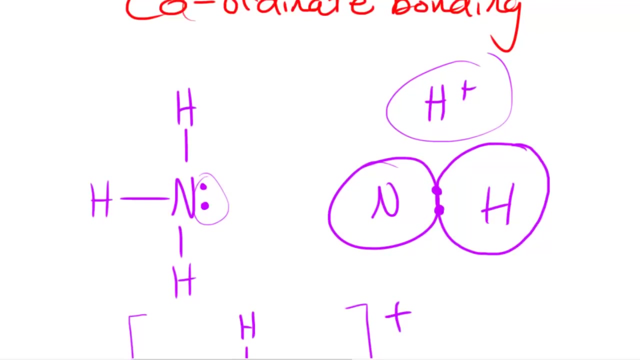 of is H3O plus ions, And the reason why this forms is the same reason why NH4 forms, because this lone pair of electrons, how it was here, these are quite negative and the H plus ion is positive, And so the H plus is strongly attracted to the negative ion. 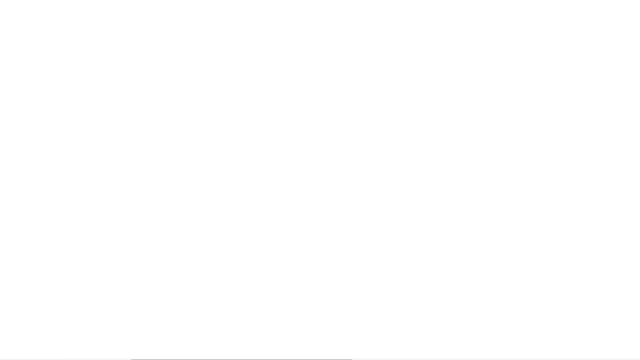 a lone pair. so if i was to draw a diagram of what oxygen the h2o would look like, so in as an equation, what it would look like is that h2o, h2o. my pen seems to be acting strange: h2o plus h plus whoa, whoa. why is it? i don't know why it's acting strange. let me just rub this out. 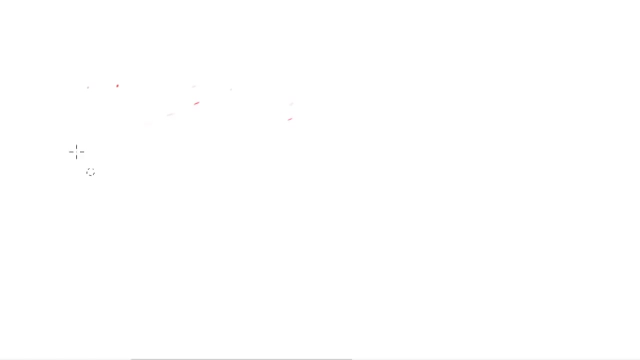 so h2, h, h2o would react with the h plus and that would produce h3o plus. and if i was to draw now the actual what, what, if you, if a representation with the molecules, we would have the h we will have. well, we'd have oxygen. and oxygen has two lone pairs of electrons, uh, not just one. 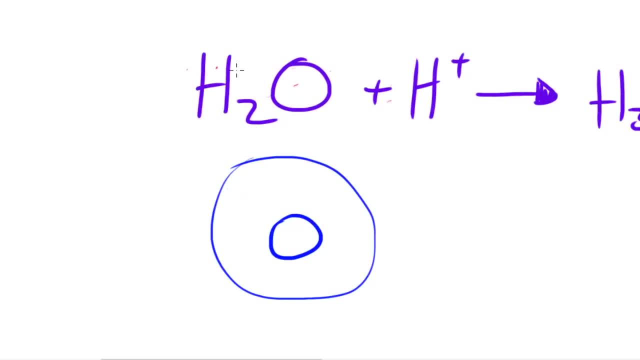 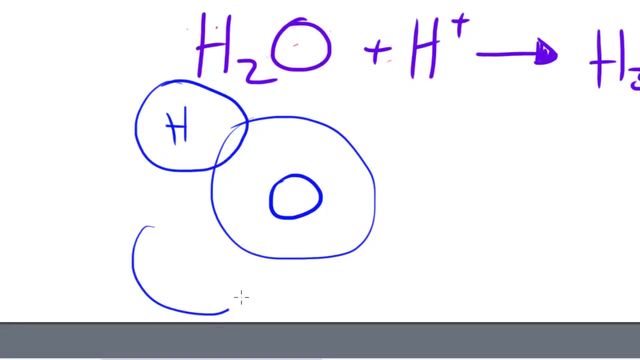 but the form? if it was to accept two protons, it'd be extremely, extremely unstable. so it tends not to form that. so we'd have um, hydrogen, uh and the lone pair of electrons. so we'd have blown pair, lone pair, and sometimes, if i was to